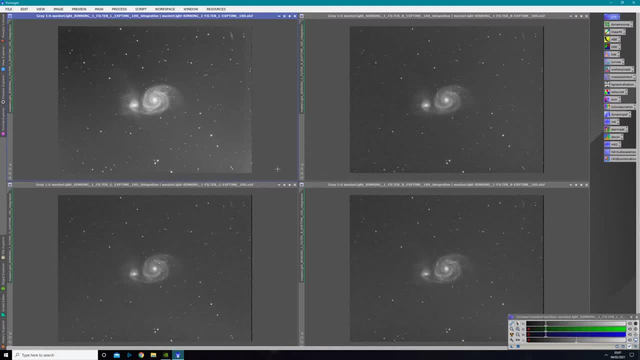 basic files themselves. but I'm going to go ahead and do that, and then I'm going to go ahead and rotate myself around a little bit thesalmanis to find relationships, and I'm going to do that through the central terminal because at the very close end of this buildings on this pictures. 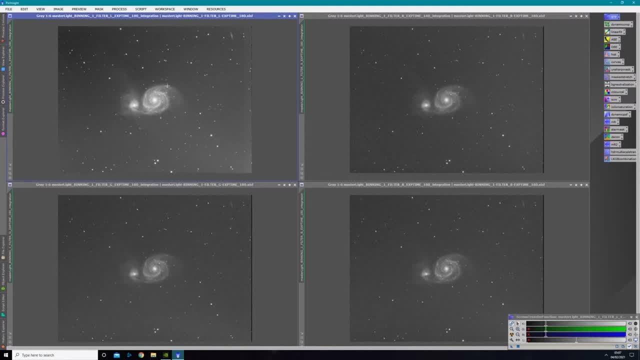 ать a real boundary with building. we don't need a big tamanants up, you just need at least a few vertical bars to be able to manage the such course. it'll probably see, on this luminance image in the top left is staking artifacts alongside a little along the bomb, not so much in the top and 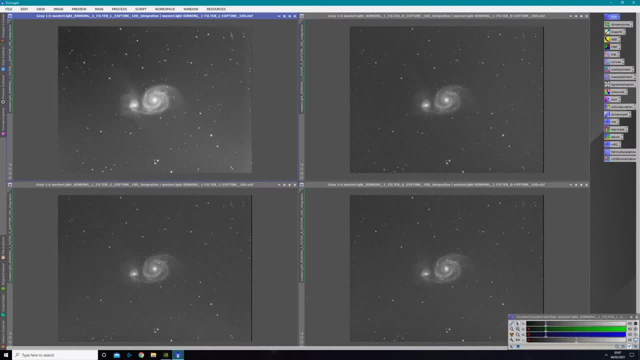 line up as they should and you don't have kind of staggered stars etc. so the first thing we want to do is want to get rid of all that by using dynamic crop so which can take in from the edges. try and get rid of the whole amount and leave none of it visible. so let's get rid of the right and the 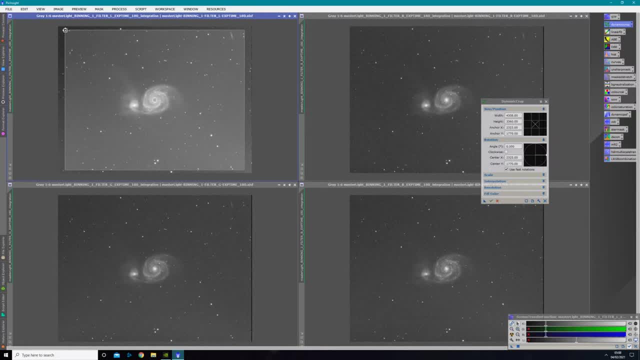 bottom. i'm going to take the left and the top until this center marker is centered on my object of interest as well. now, rather than just clicking tick, which is only going to apply this process to this particular highlighted box, i first want to apply this exact same crop to all my other. 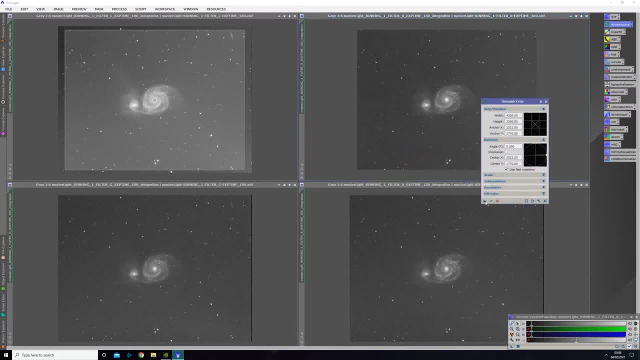 registered images. so you do that by dragging and dropping the little new instance icon to the other images first. now that's done we can go ahead and click and apply it to the main image. so the next problem we can see straight away on this luminous image is quite a strong gradient. this is, i mean. well, i say strong, it's not too bad. 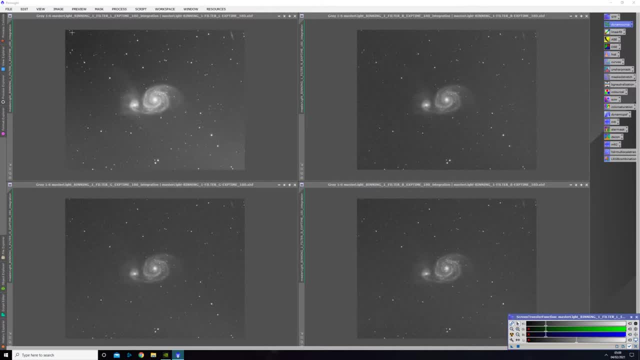 but, um, you can see it's lighter in the bottom right and darker in the top left, kind of going fairly evenly across the the field of view. now i'm going to try and get rid of this with a dynamic background extraction, so what you need to do is place a few modeling points around without 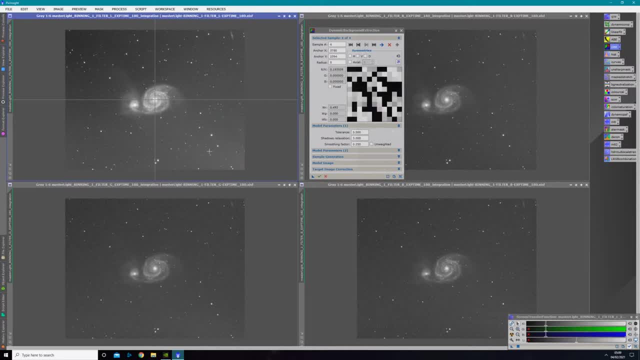 selecting stars or galaxy to effectively let this create a mathematical model as to what the background should actually look like with these gradients subtracted. so let's place a few of those. you don't really need to go crazy, you just uh, perhaps 20 samples or so is enough to get a good model created. well, we'll soon find out. 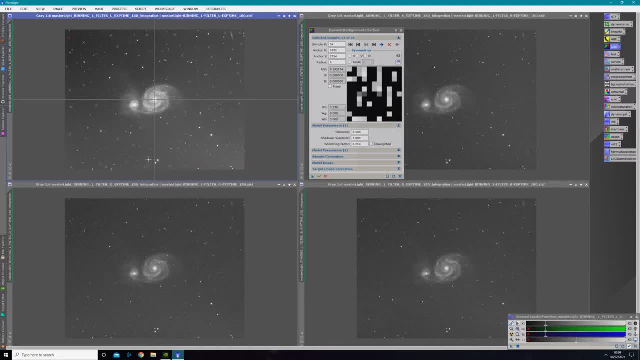 and i'd say that's about done. so. the target image correction- so this is the target image and the correction i want to apply- would be a subtraction, and in this case i'm going to discard the background model. but all that does is, once you've applied this to the image, it basically just shows you what was subtracted. 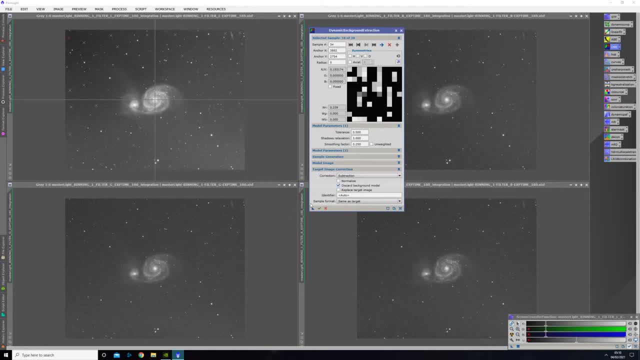 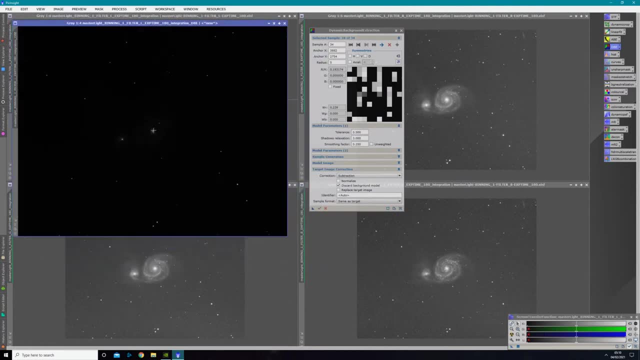 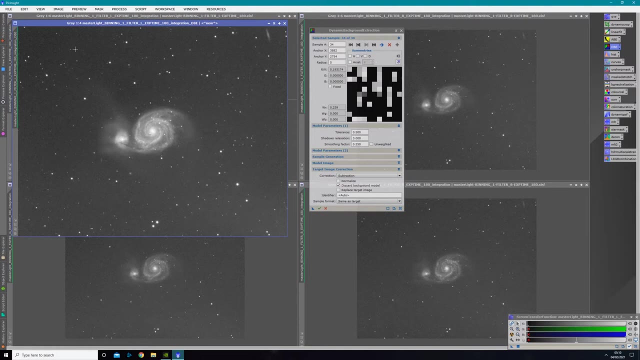 which is not really needed for this. it should be quite an easily removed gradient. we'll soon see. so it's now got this one selected for us and, as you can see, it's been returned to a fully linear state. so we're going to need to apply another screen transfer function and, as expected, 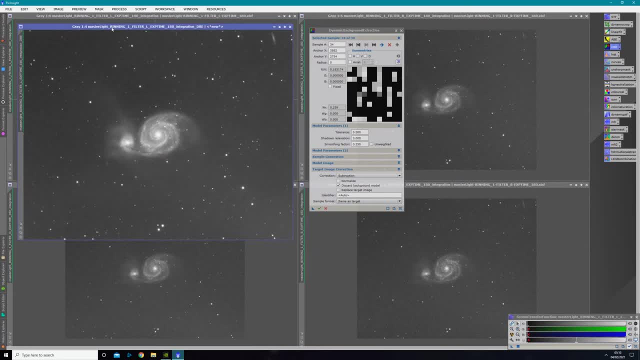 almost all of the gradient in one pass, but it's not quite fully gone and i think the model still is valid, so i'm just going to go ahead and apply that again, this time to the newly created image screen screen transfer function. again, and yeah, that's definitely better. so go to end that session. 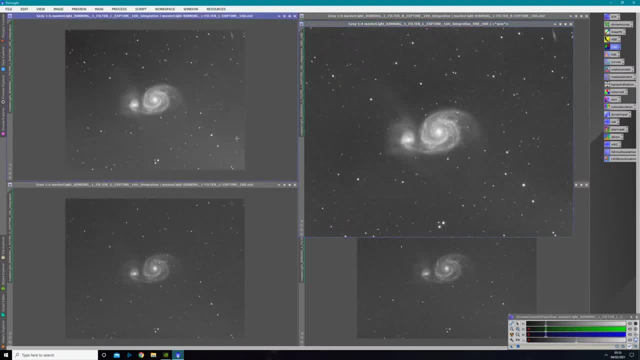 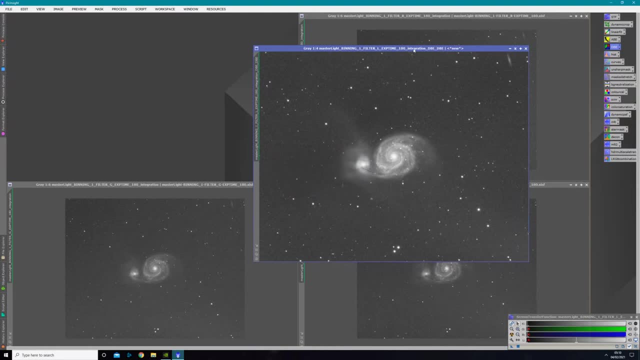 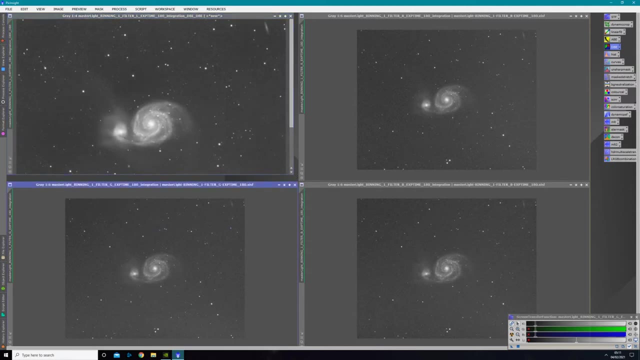 close the uh other versions of this image just to reduce clutter on the screen. so i don't need this anymore. so i'll close that and move that there. so i want to do the same sort of thing to these, but, as you can see, the gradient is much lessened. i think this is because it was shooting through. 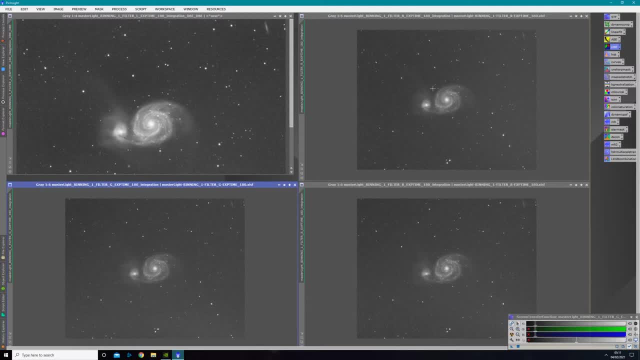 individual colored filters- green, blue and red- and they cut out a lot of light pollution that gets through on just a luminance image which makes gradients far more noticeable, always on that channel. so we're going to start with the green first and because it's such a gentle gradient, i don't think 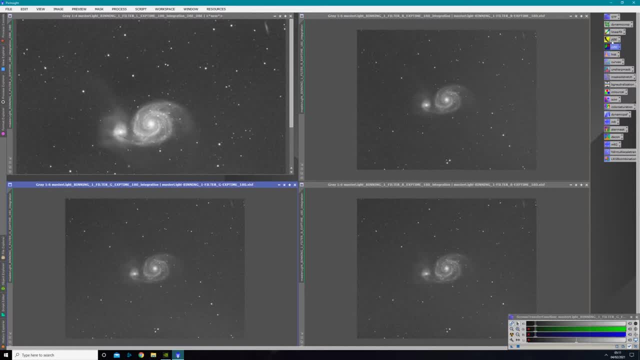 there's any need really to use a dynamic background extraction and i think we could trust the automatic background extraction tool to work. we're going to need to apply the same correction, which would be a subtraction, and also we want to get rid of the background model and we could just drag. 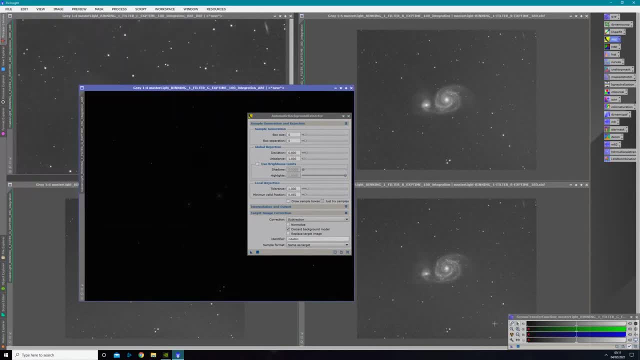 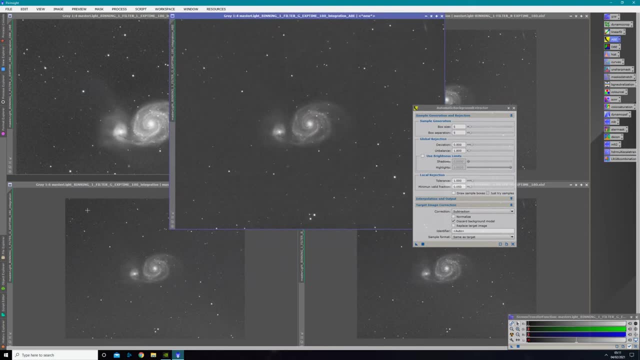 that and drop it on top, check the result and, as you can see that the the very gentle gradient is now all gone and it's largely flat, which is just what we want. so i'll now close this one. i'm going to do the exact same thing to just these other images, so i'll do it to red now. 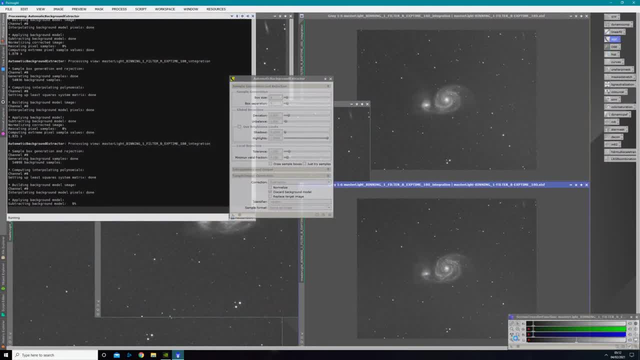 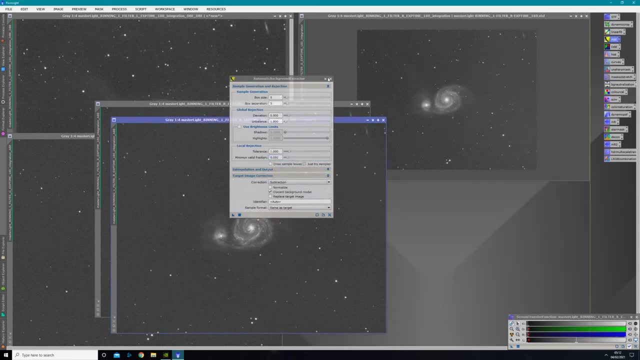 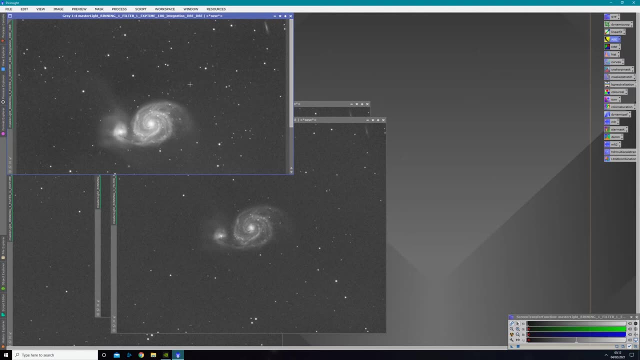 and to blue and i'm satisfied that they're all corrected. well, so i'm gonna go ahead and close the original gradient originals just to reduce clutter. as I say So again, I want this one in the top left. they've all ended up stacked and cluttered. I'm going to go to the window tool and tile. 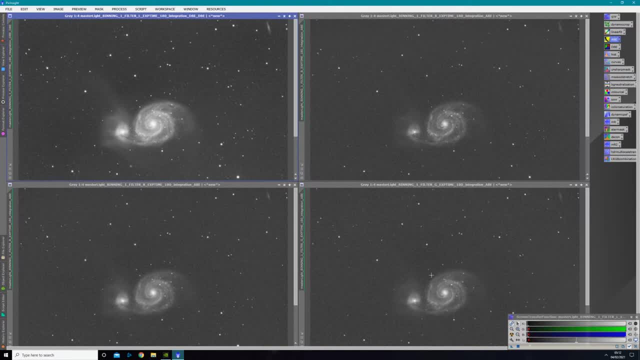 them again. So now they're all lined up neatly. The next thing that we could do is basically apply this screen transfer function, which looks quite good, quite good level of stretch, as it introduced too much noise in the linear phase of the image, and we're going to apply. 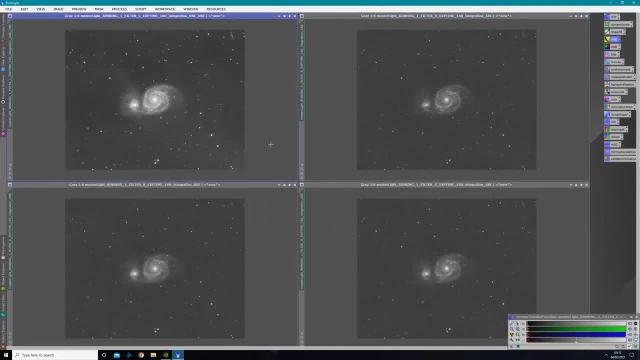 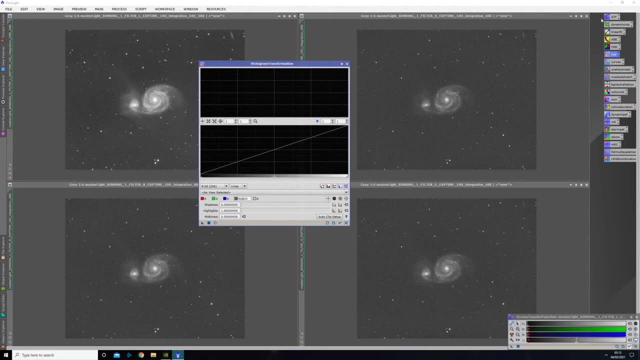 it and make the image non-linear, ready for combination. So how to do that in this program is basically open your histogram tool. I already have a list of processes I use frequently lined up at the side here. You won't have those unless you've done them yourself, so 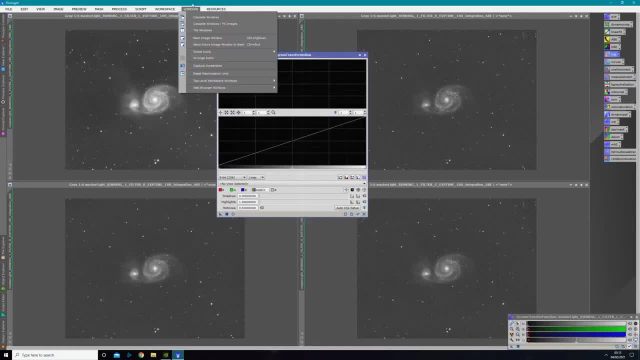 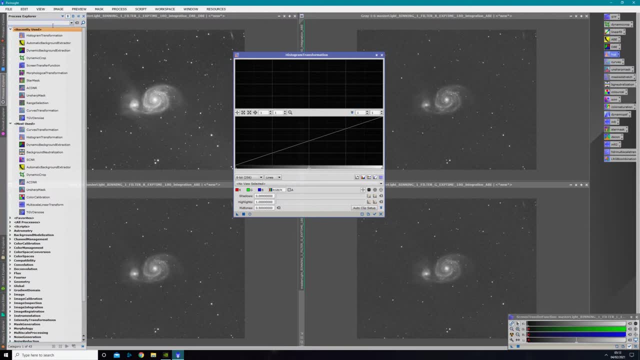 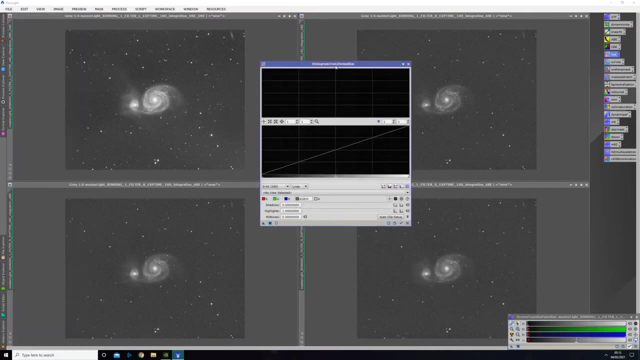 you'd have to manually navigate to each one of these, but they're not too hard found, and also it's worth mentioning that there is a a search box on the Process Explorer, so you can just type histogram and there it is for you, But anyhow. so I want to select the image I'm going to work on, drag across the STF. 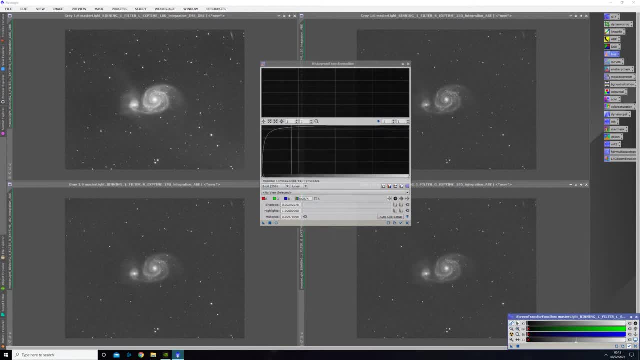 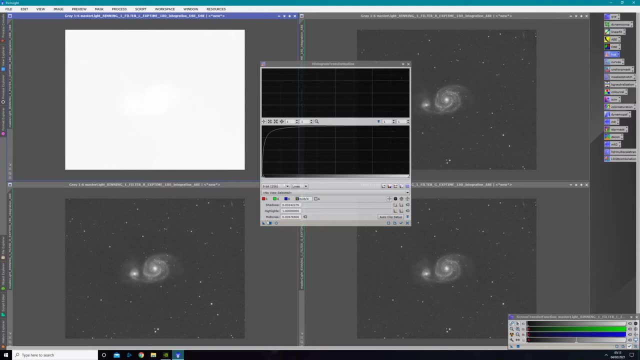 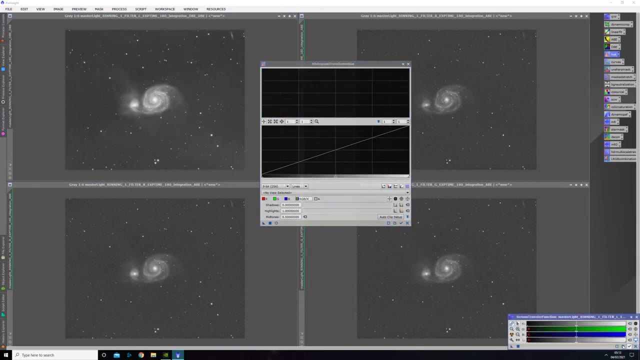 to the bottom of the histogram tool You can see. now it's going to show you where it's histogram is placed and then we're going to drag the histogram itself, the apply button, from that onto the target image. I'm going to go ahead and reset that and reset the STF, which is now no longer being. 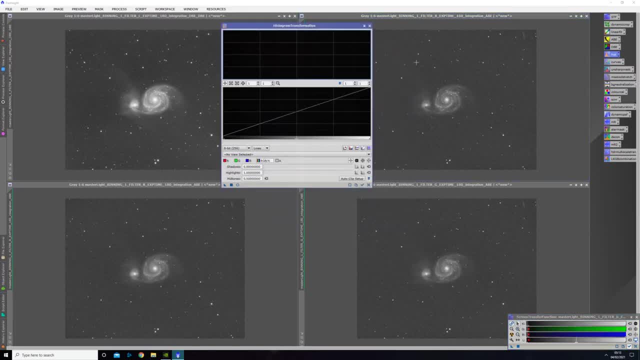 applied and perform these same steps for each image. So blue: drag the STF to the histogram and the histogram to the image, Reset both and move to the next. So green again histogram to the image And once more the STF panel to the histogram, to the image. 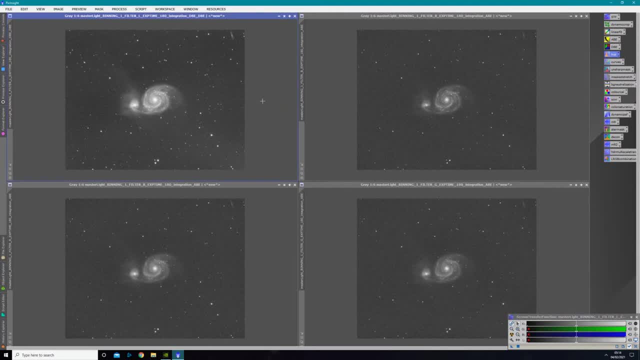 So now we've got all these images in a nonlinear state and that's the best time to combine them. basically, then, We're using the LRGB combination tool into a full color image, So we're going to go ahead and select that L is the image we want for the L channel. 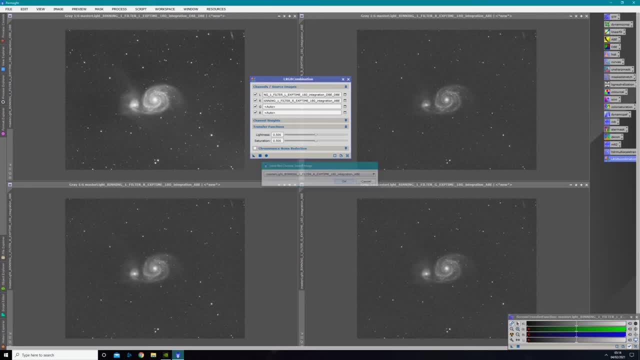 R, of course, for R, G for green And the B for blue. And I am going to go ahead and apply some chrominance noise reduction to this. Chrominance noise is just your color model. effectively, It should leave largely the galaxy alone, as the signal is so strong. 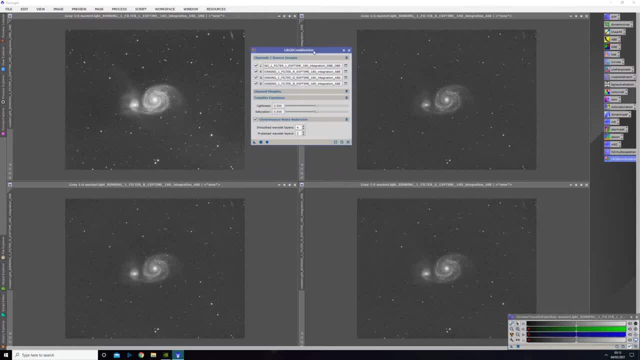 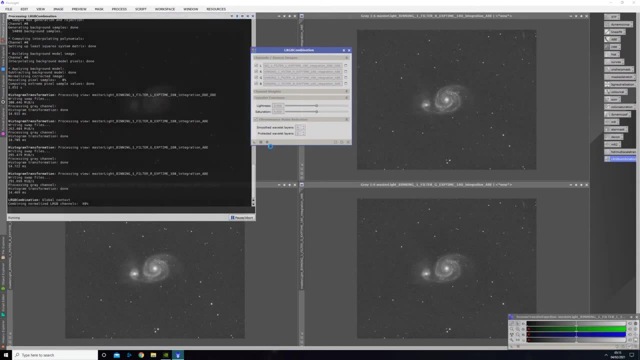 in that area. It shouldn't be very effective. It should leave largely the galaxy alone. as the signal is so strong in that area, It shouldn't be very effective. It shouldn't be very effective. It shouldn't be very effective. So we're just going to go ahead and apply global 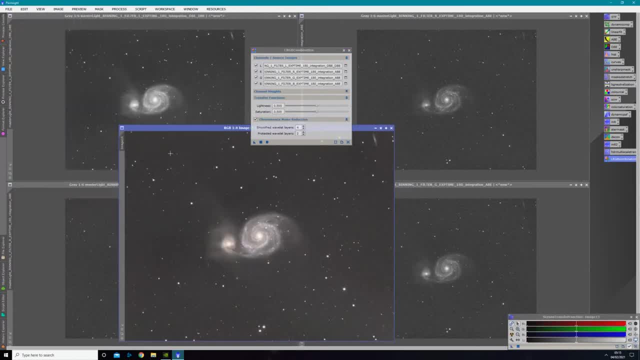 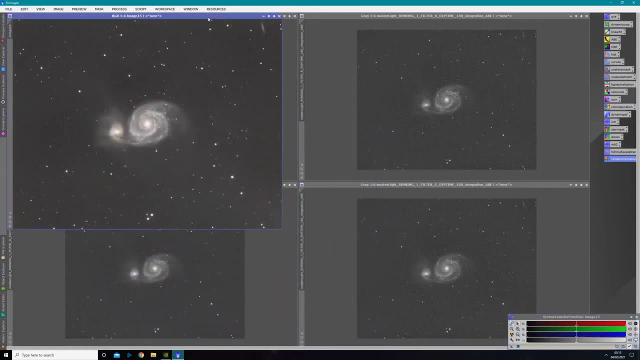 And it should just take a moment. OK, that's done, So we can close the LRGB combination tool. now Move this into a workable position, And I'm also going to take the image identifier and drag and drop it to make a clone. 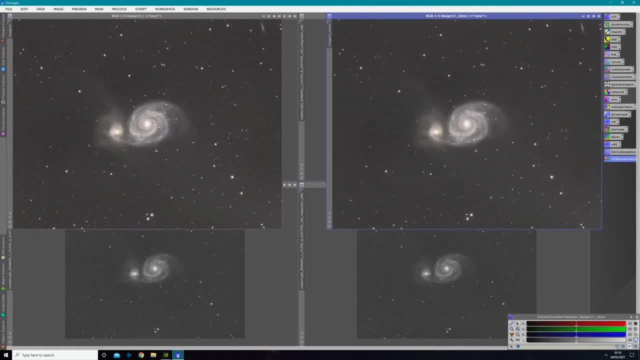 And we're just going to move that across to one side for a moment. we can see where we've actually came from In the background. I can minimize all these to reduce some visual clutter. Okay, so we're going to be working on this image Now, the first thing I'd like. 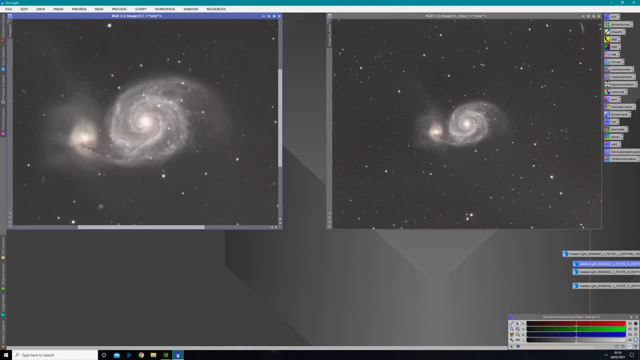 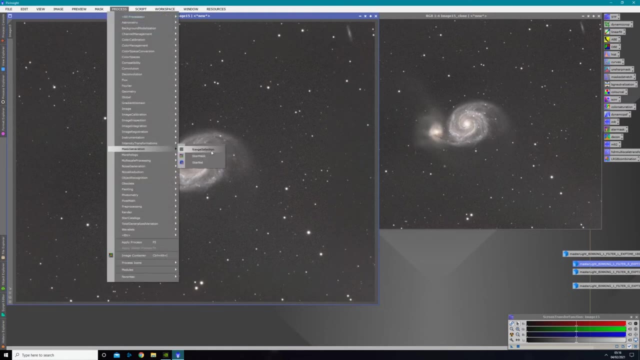 to do is to denoise the background ever so slightly while leaving the galaxy alone. So to do that, I'm just going to zoom in ever so slightly on the preview and we're going to open process and go to mask generation and I'm going to 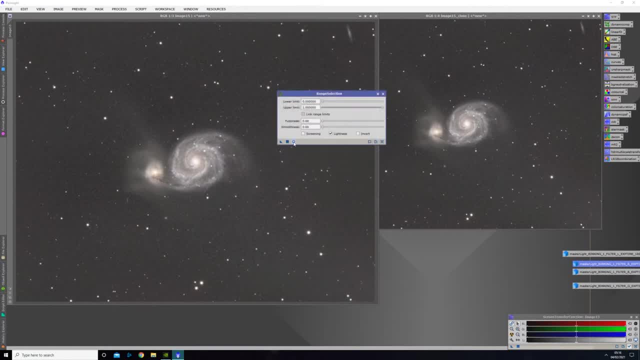 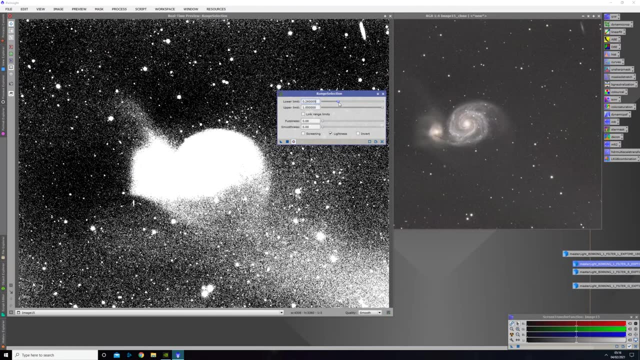 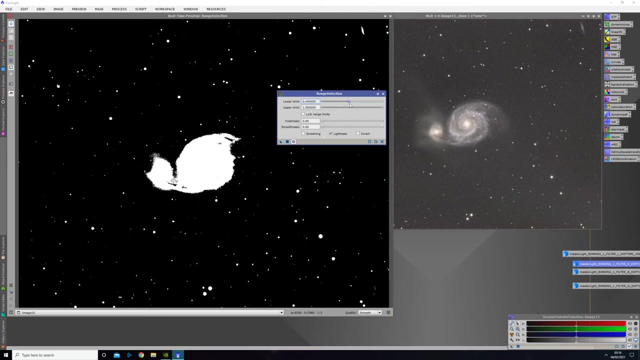 create a range mask. This little circle will allow you to preview what the mask is going to be and if you bump up your lower limit, you'll start to see the actual target that you want appearing. So I want to be picking out mainly just the galaxy and leaving the background alone in this, and 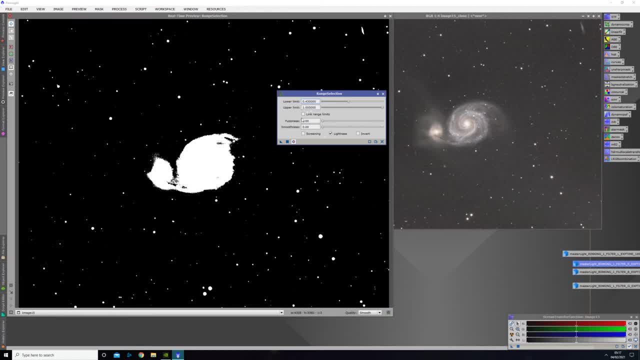 about that sort of selection should do it. There's still a nice separation here between the galaxy and the background, just as there should be, as you can see on the cloned image, and I'm not going to invert this just now by using this, because I'll show. 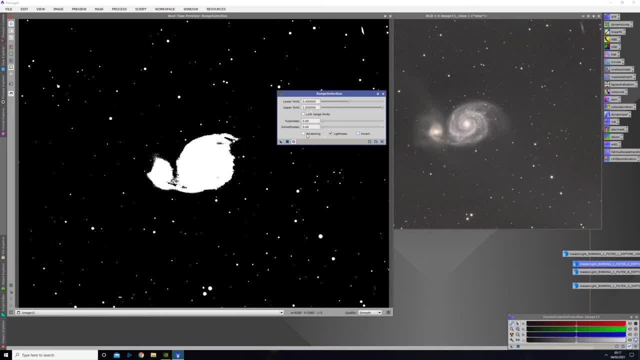 you. there's another way to do it. we can just use this one mask for just about everything. I am going to apply some smoothness either, so that the transition from the process as I'm performing are going to be smoothed out into the background and not be quite so stark. 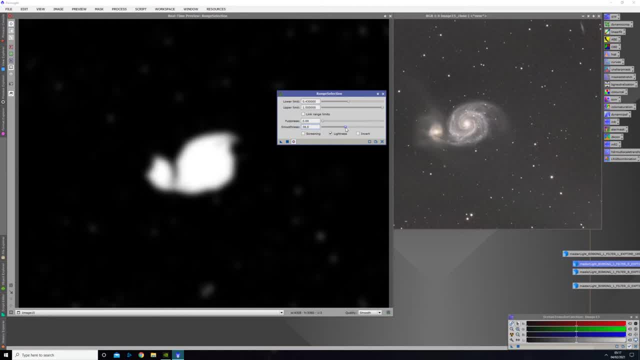 edged. So I think around about there looks good, we can still see this subdivision, because I don't want this section not to be noise-reduced, otherwise causing a little pocket noise right here, It will look bad. It will look bad for this hand. 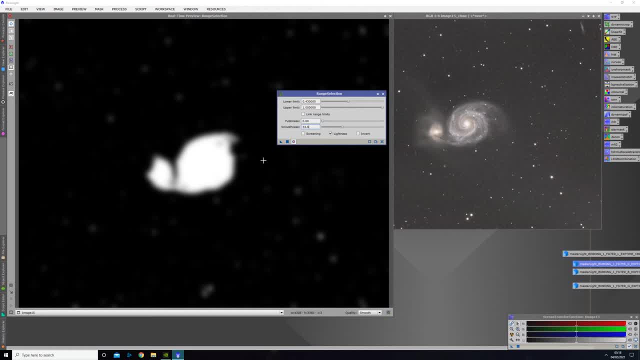 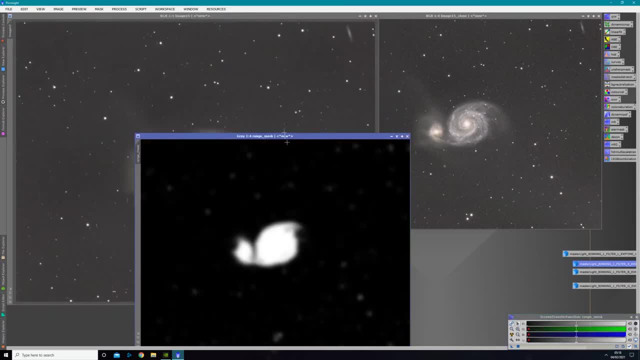 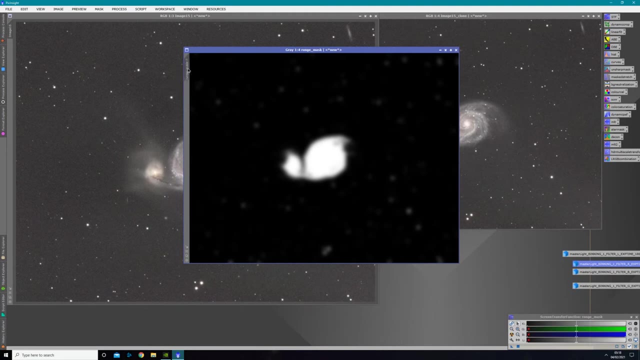 little pocket of noise right there. Alright, so we're going to go ahead and apply that. We'll close this and close the preview. and now we've got a range mask. So to drag and sorry, should I say to apply a mask in PixInSight, you can. 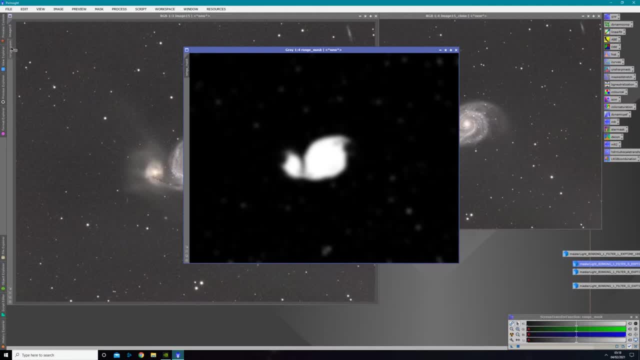 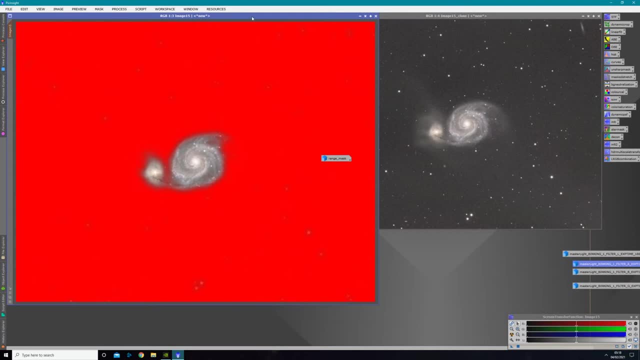 just drag and drop it just below the image identifier of the panel you want to apply the mask to. I'll just minimize that for a moment now. It'll still be in use as the mask, as you can see. So currently the masked area is the. 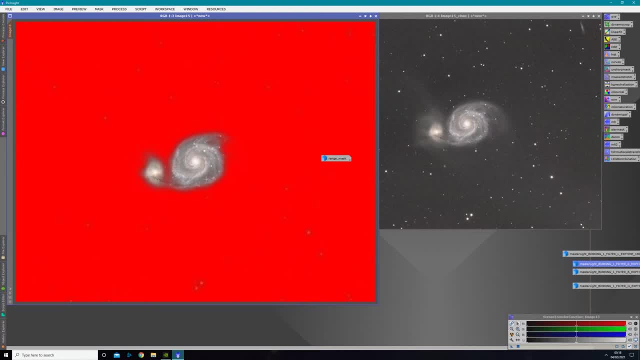 background and I actually want to work on the background and protect the galaxy. so this mask needs inverting. We can do this by just right-clicking going to mask and selecting invert mask. So that should be the galaxy nicely protected and all the background ready to be worked on. So I've been 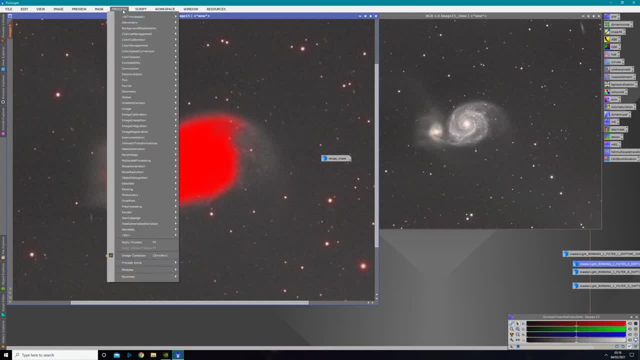 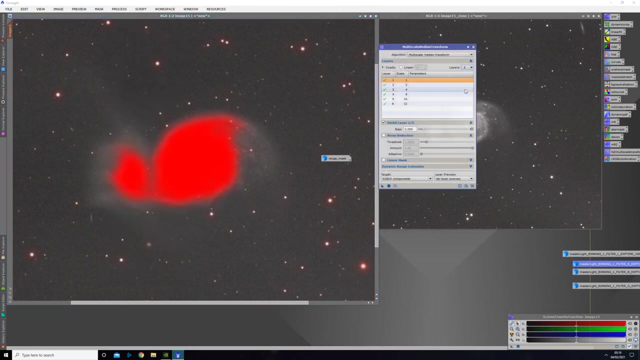 experimenting with noise reduction for easy image processing that's performed in the nonlinear phase. Usually you do noise reduction in this program while the image is still linear, generally using multi-scale linear transform, but instead I'm going to use the multi-scale median transform, Up the amount of available layers to five We. 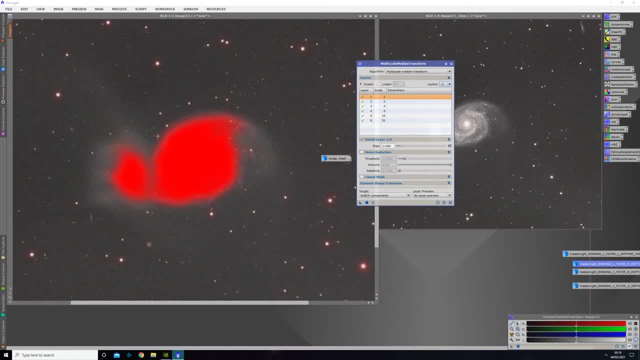 don't need a linear mask, because we've already got the masked part that we don't want to work on. so we've already done that ourselves. so, with no need for the, the masking tool, I'm going to apply noise reduction on each layer in largely. 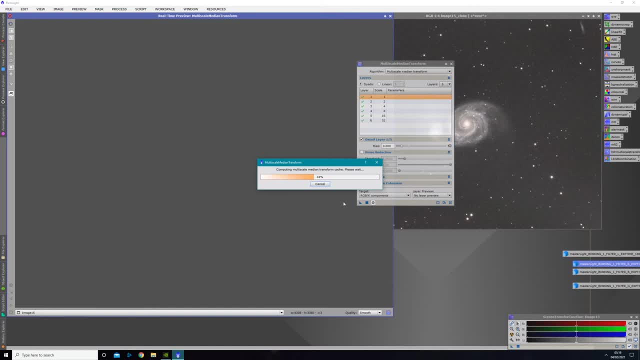 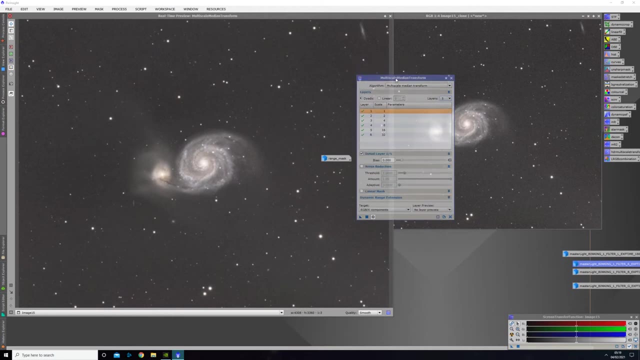 similar amounts, just to keep it simple for this tutorial. I mean, if you're working on your own image, you probably want to take far, far longer than this and go much more carefully and ideally, apply and undo, and apply undo and see the effects that you're having on your image. 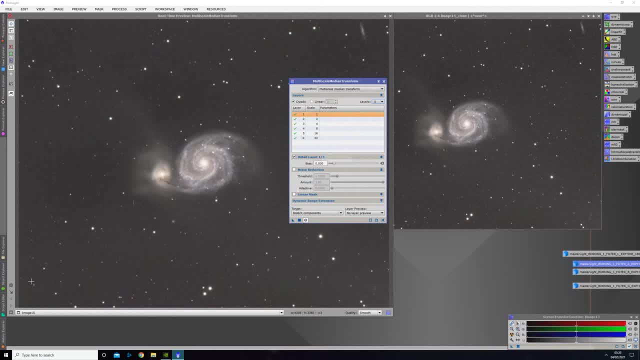 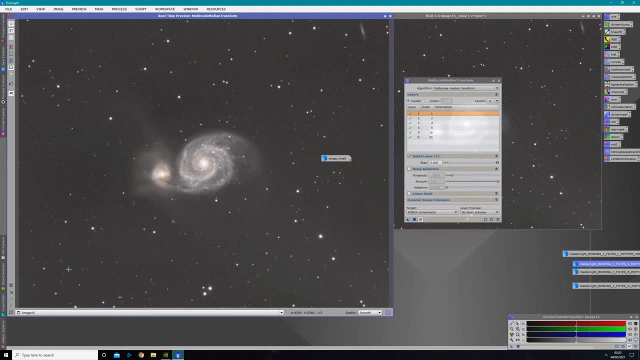 But since this is just a quick tutorial, if I just go ahead this way. So now we've got the preview window open again, by selecting the little circle I want to actually drag a new preview window across a region of interest to the galaxy. so I want part of the galaxy in the view and part of the background. So 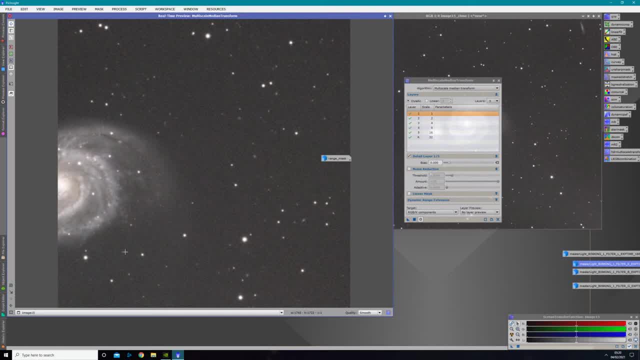 now we can hopefully see that when I'm applying this noise reduction, the galaxy is left alone and the background itself is the only part being denoised. So I'm going to apply this noise reduction and the galaxy is left alone and the background itself is the only part being denoised. 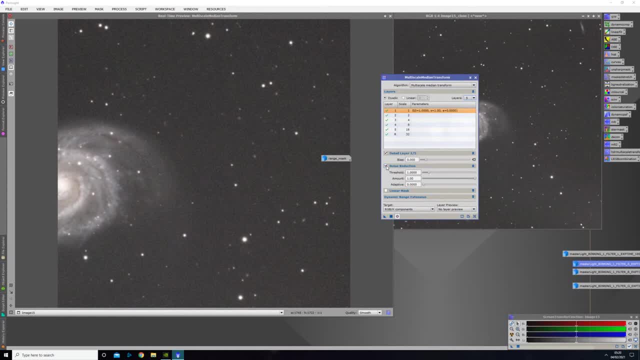 So I'm going to enable noise reduction on layer one and apply a middling strength. Same thing layer 2. layer 3 gradually getting ever so slightly weaker as the layers are gone generally. You can already probably see it started to denoise it's. 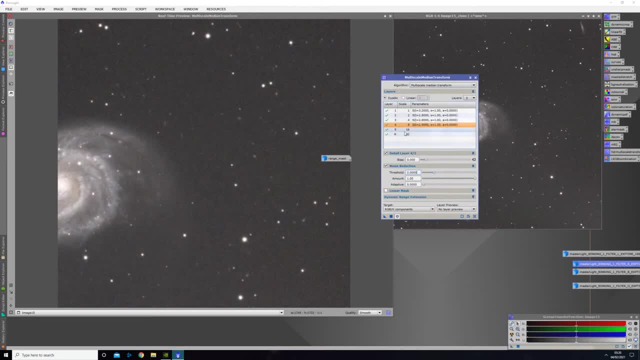 background. quite well, try it on about two there on this last layer just a little. So if I just show the transformed image and the knot a couple of times, hopefully you can see on your screen the effect that that's had. It's left the galaxy alone just. 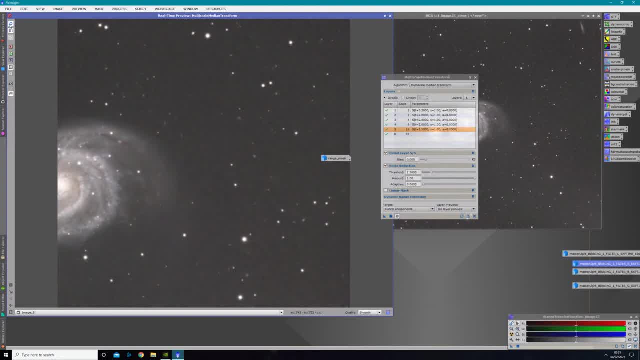 as we'd hoped, The background is largely denoised. it's looking quite smooth. There's still some chrominance noise, as in colour model, and there's also kind of a salt and pepper noise appearance to it, but we're going to remove that in a moment, So I'm going to go ahead. 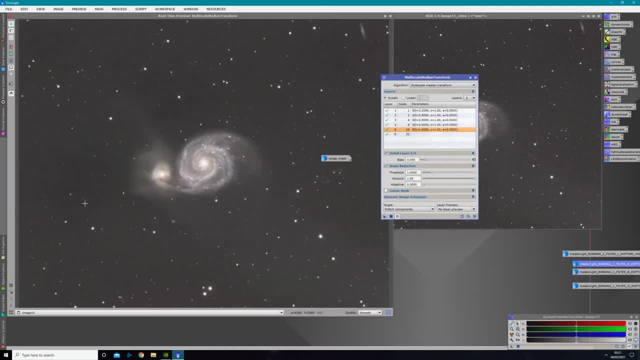 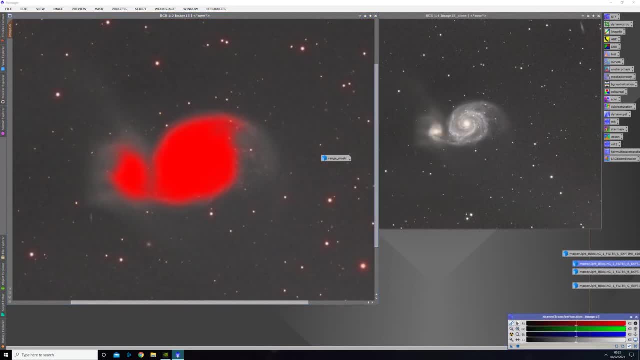 and apply that. Okay, and that's finished, So we can go ahead and close the preview, close the media and transform tool, and now we're going to address that background model. So the tool we're going to use for that is found here. so it's process noise reduction. 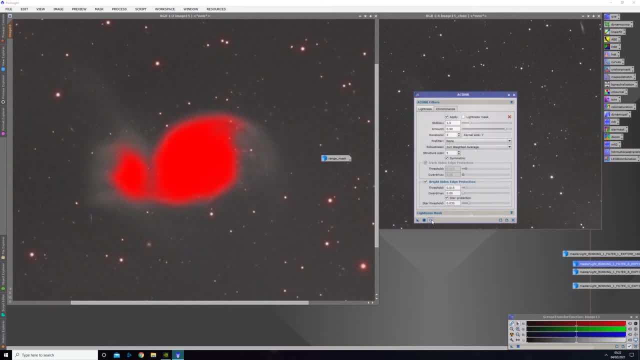 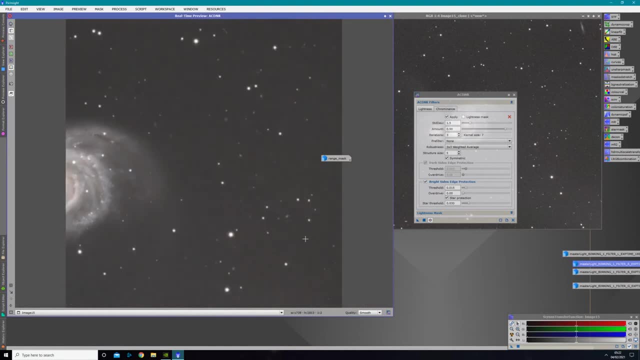 and ACDNR. We're going to again open a preview, open a region of interest, and this time we're going to not use the lightness mask again. I should add: We're going to apply just a little of this because that's automatically. 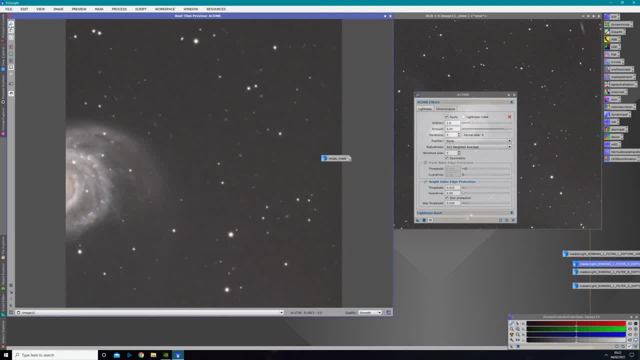 getting rid of all that salt and pepper noise, And by salt and pepper noise I mean kind of a black speckle that's over the whole image and hopefully that's showing for you that that's there and then gone, While leaving the galaxy alone. 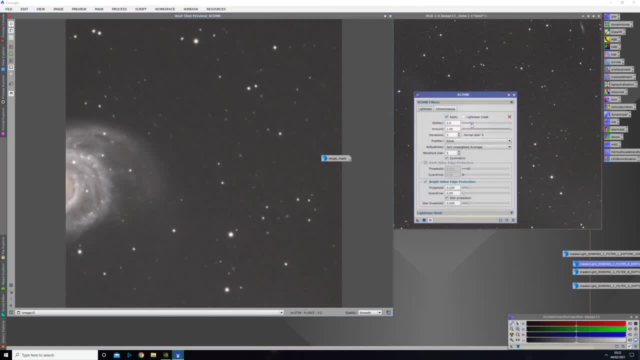 So I'm satisfied with that. However, I am going to apply a small amount of chrominous noise reduction. I don't want to overdo this, because it will take any color that's left out of the stars, and we don't want that. So just a small amount and then apply. 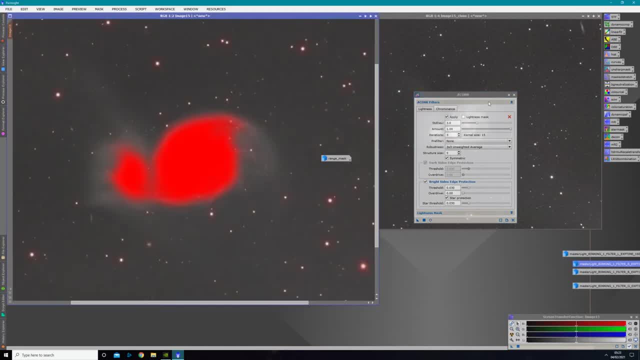 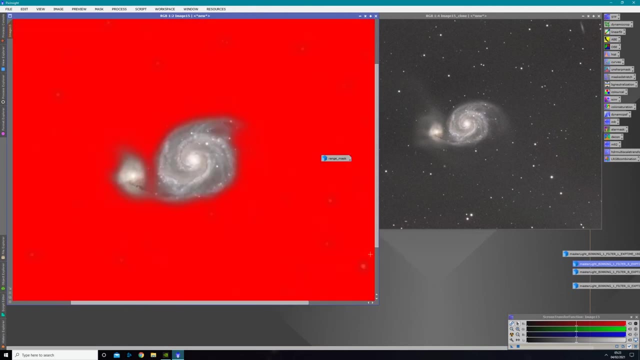 Okay, that's finished. So we're going to close down our tools and I'm satisfied the background now is largely smoothed and worked onto an acceptable level. So now I want to work on the galaxy itself. So this mask, I'm just going to invert it again, put it back to normal. 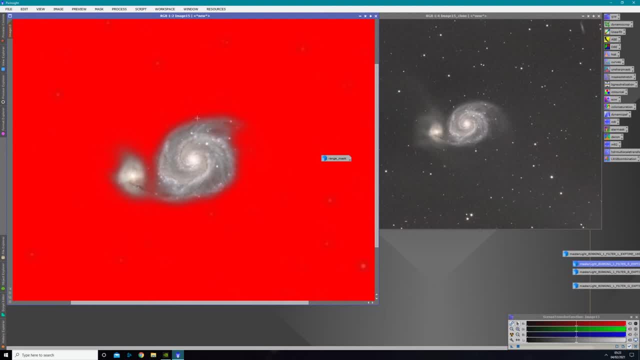 So before changing masks and risking applying a new range mask and leaving sort of a ring artifact where the masks don't quite match, I'm going to keep using the same one and just apply a light passive noise reduction to the galaxy itself using TGVD noise. Now, we don't want this to be too powerful and start ruining detail even. 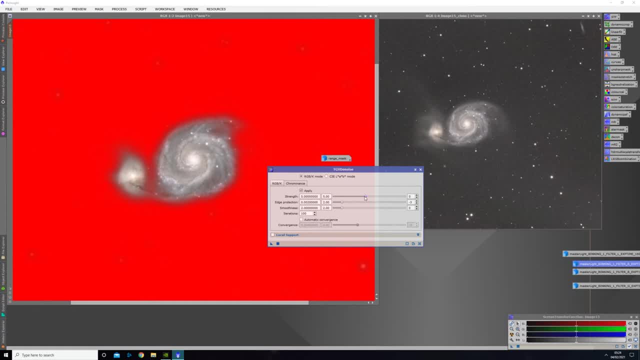 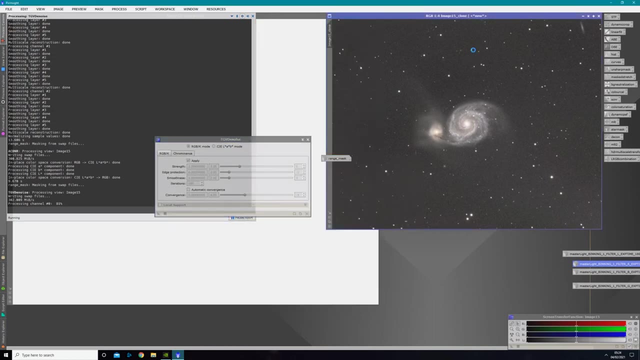 though this tool itself is very good at preserving detail, So I'm just going to turn it down a little to around 3, 3.5, and I'm going to apply that. It would probably be useful to mention at this point too, that, well, that's processing On your own images when you're 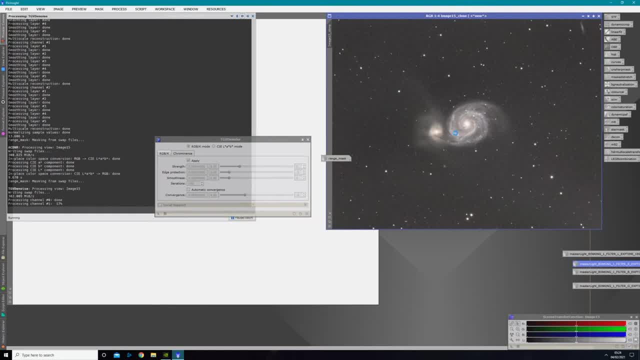 taking your time doing this, you can actually preview what the effect would be without waiting for the whole process to occur on the whole image. And you do this by holding down Alt and pressing N, And with that you can draw a preview window once it's done processing. 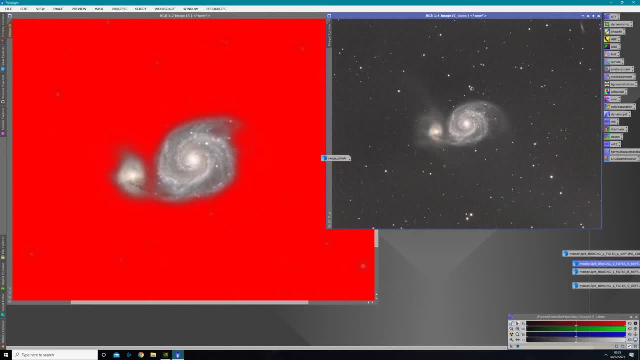 Alt and N and it brings up this little icon. And now you can drag out a preview window and it will be put just below the main image identifier for you. So just to give you a little bit of an idea of what the process would look like. I'm 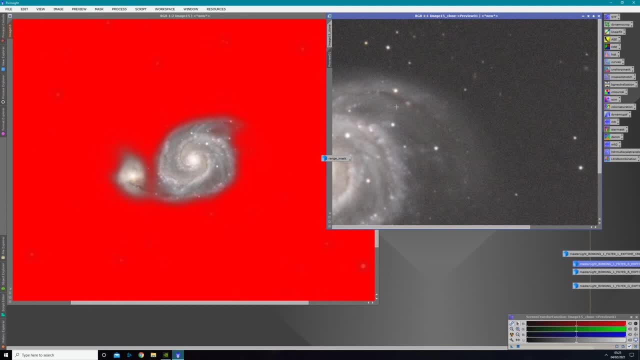 going to go to this. You could have applied any of those tools and it would have been non-destructive to your actual main image until you were satisfied with the effect, just by going, you know, Apply Undo, etc. On this tool you can only ever apply one modification. 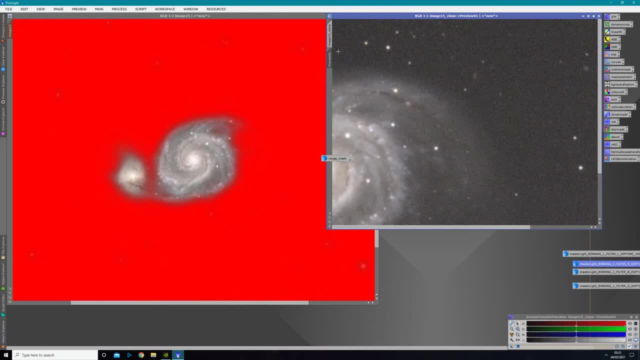 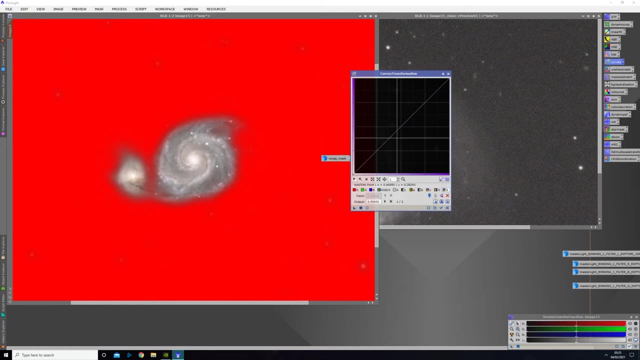 to a preview at a time. You can't stack them, So that's worth noting. Anyhow, back to the main image. So we're going to keep this range mask as is and apply that. I'm going to apply some curve transformations, So I want Saturation, which is this end tool. 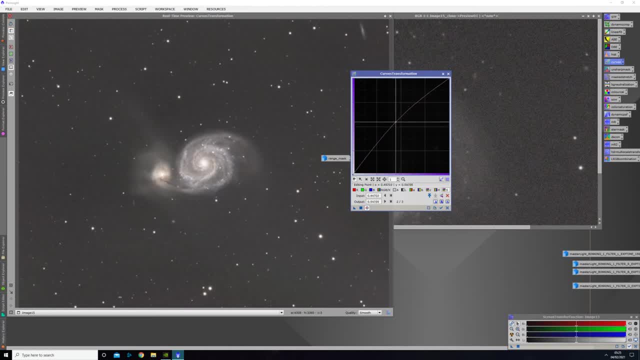 a preview, And I'm going to just gently bring it up from the middle a little until we can just about start to see some color appearing. Hopefully you can see it looks almost monochrome there and then starts to get some color. Don't want to go too far with this just yet, so I'm going to apply that and leave her at. 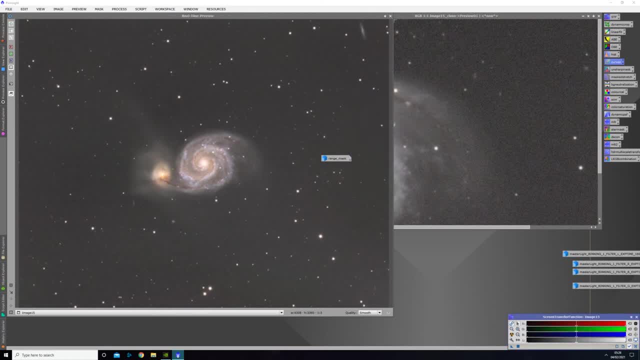 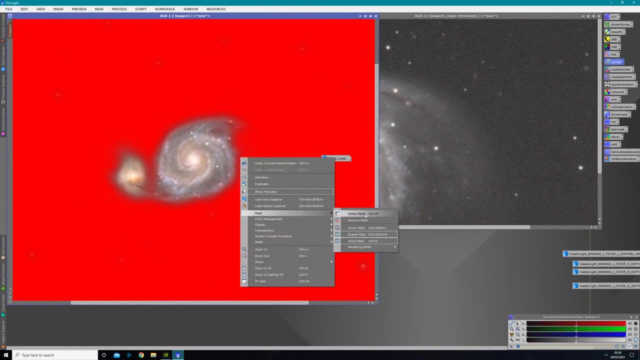 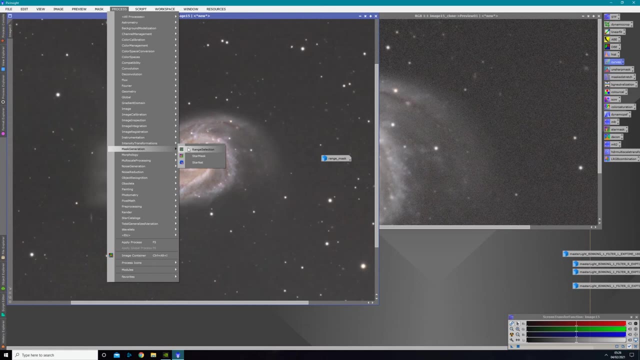 that. reset the tool. close that. close the preview. at this point I'm actually going to remove this mask and make a fresh range mask. I'm gonna do this now so I can actually be a little more inclusive of the fainter regions of the galaxy. so 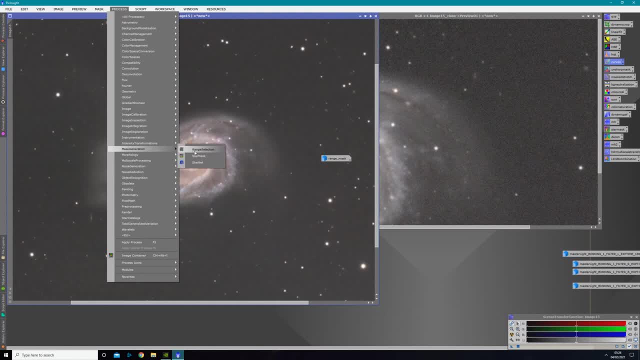 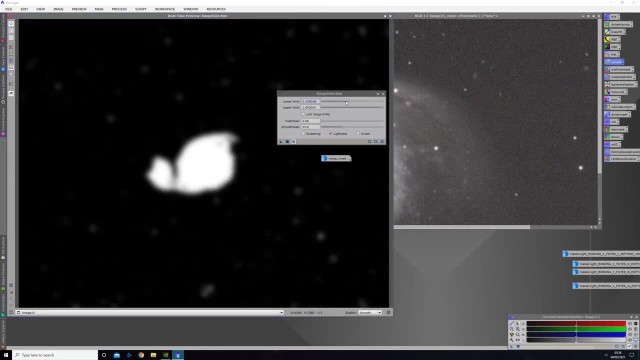 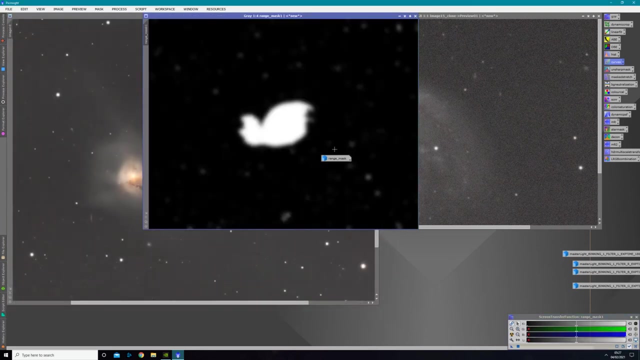 again: process, mask generation and range selection. you can see that was the parameters for the previous mask. this mask I'd like to be ever so slightly larger. I think that'll do it, so I'm going to apply that, close the preview and move our old mask out of the way. 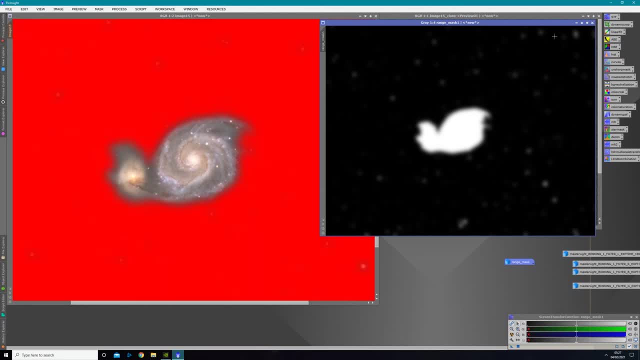 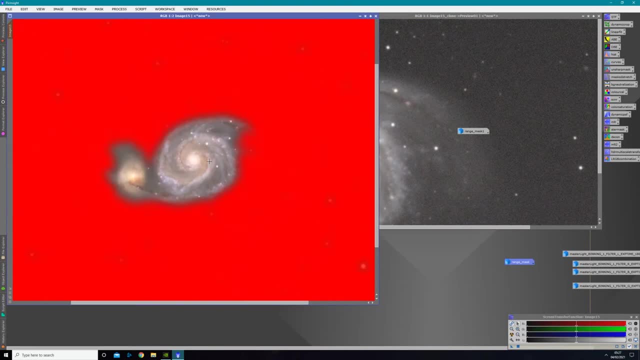 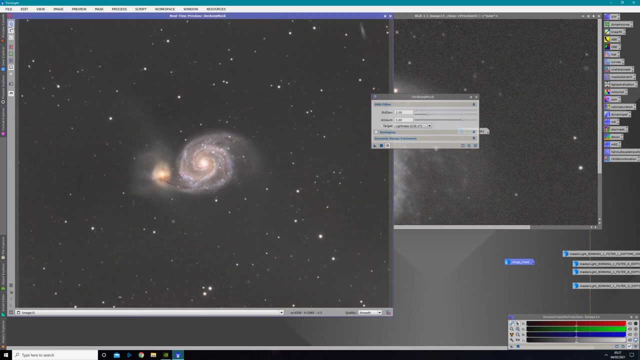 and drag and drop this onto the image. okay, go ahead and minimize that, so it's looking quite good. we're also fairly soft, so I think a small amount of convolution and unsharp mask will help rectify that somewhat. so, as you can see, even with the- just the defaults, that already looks better for just to close. 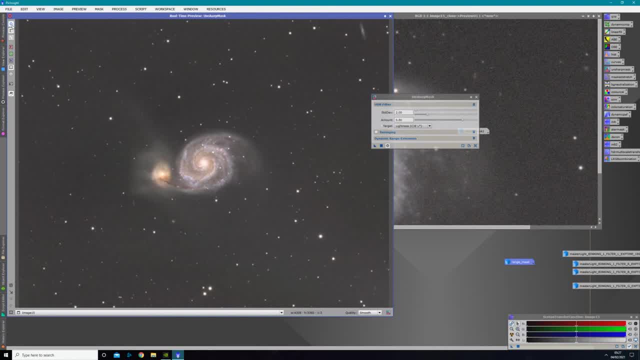 and reapply sometimes. this is one of those tools where you can really get out of hand and make a huge mess of your image, as you can see, if you just went too far it looks awful, but you can always put things back to the basic parameter like that, and I think I'm gonna stick with that, as I don't want to. 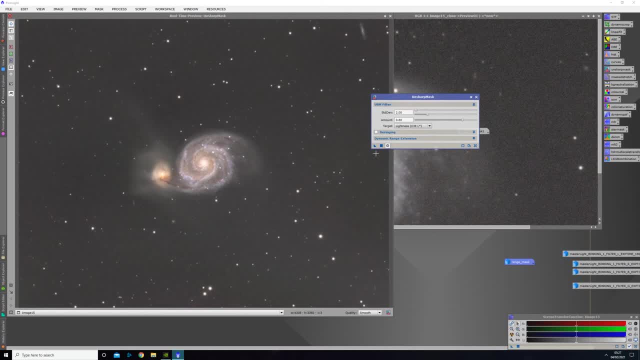 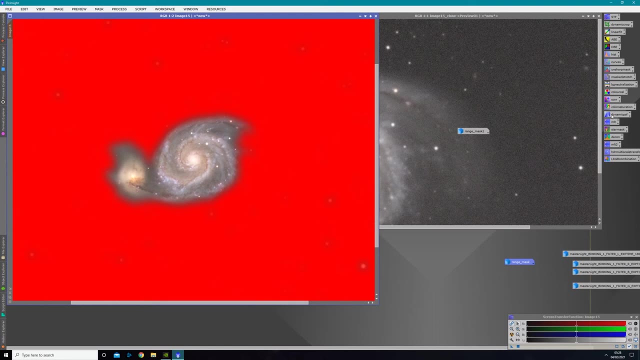 go too overboard and have things start to look a bit fake, if you like. okay, so I've applied that again. close the preview. and now, this time I want to bring out some more selective color to galaxy, so for that I'm going to actually use the color saturation tool itself. now, with this tool, you can actually hold. 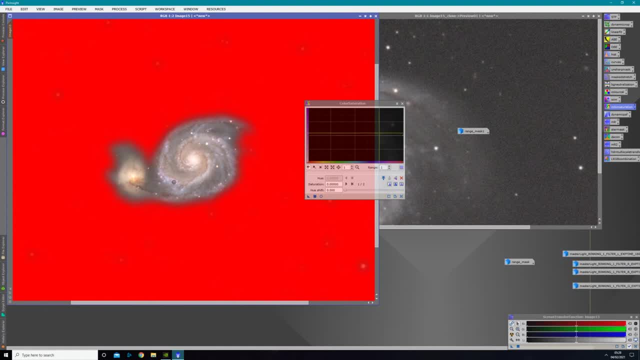 your left mouse button down on a region of the image and if you can see on the tool itself that it's showing you what color information is available for that part of the image. so if I want to bring up the blues, I'm going to select the 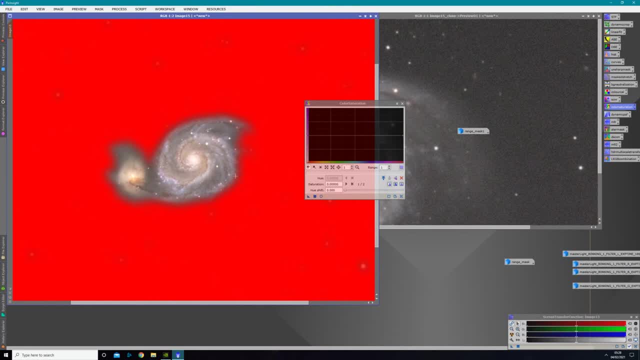 area of the images that should be blue like these, and you can see it's around here that it's highlighting. so if I just put a little pip on the histogram there and I can see it's going to be blue like this. so I'm just gonna drag it up the 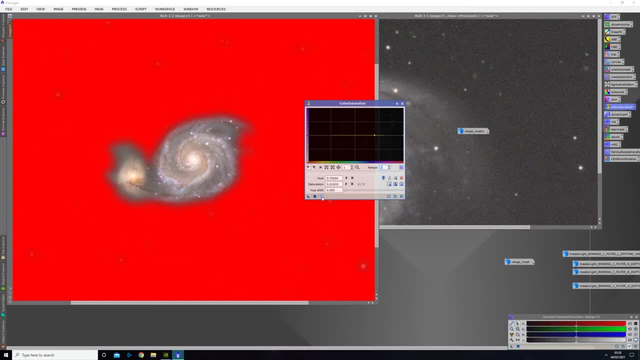 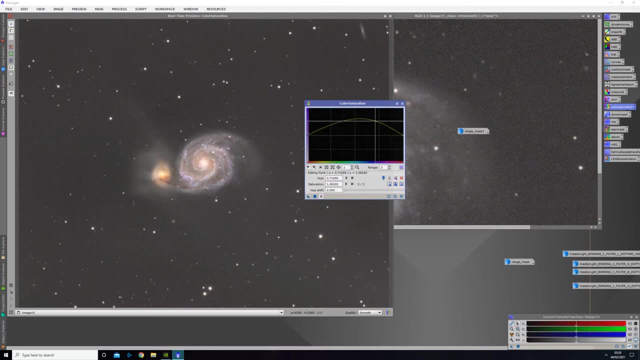 range. so the range, basically, is the strength of the transformation we're about to apply to this image, want to make a preview so you can see what effect we're having, and just drag just the blues up for now, without worrying about the other colors, until the point where you satisfied, so I'd say around. 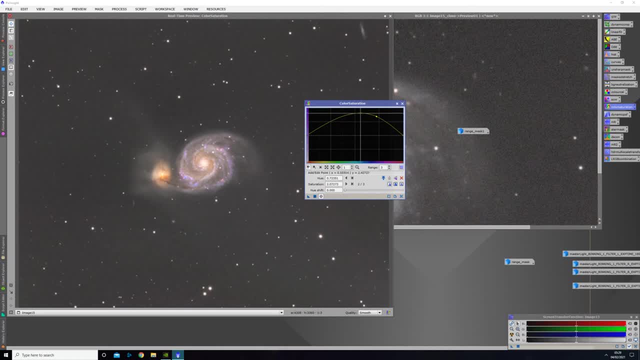 about. there is enough blue. now, before applying this, I want to actually take tool again and manipulate the color. so I'm only targeting the color I want. so, as you can see, you do that by putting little pips on the line and effectively wrestling it into position. so that's how it was. and now, with the blues bra of. 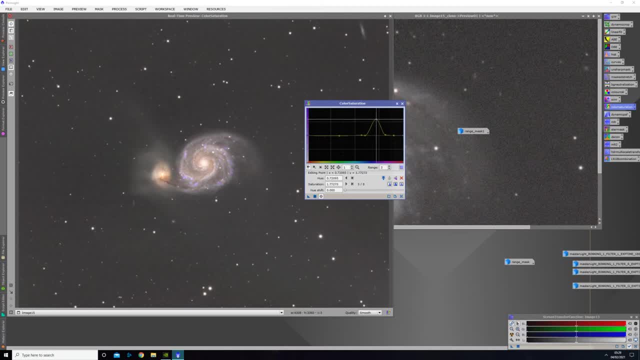 course you can go too far with this as well and have things start to look a bit pastel, but I think moderation is key when trying to process galaxy images, especially nebulae. you think you've got a bit more creative license, but galaxies, I think the largely won't leave in looking more natural, so I'm going to 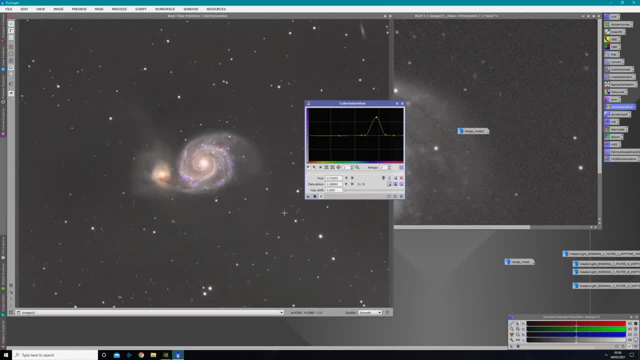 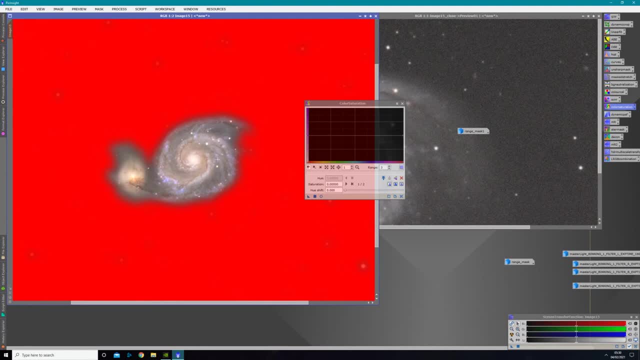 apply that reset the parameters. and now I feel I'd like to perhaps bring up some of these reddish areas- red and pink, as you can see. so they're going up here. I'm going to drag that up and drag the rest back down and roughly see the effect. 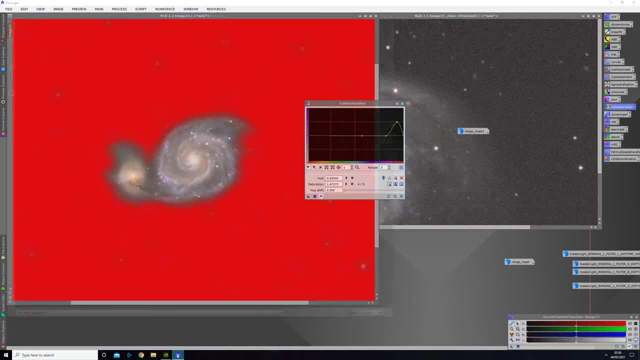 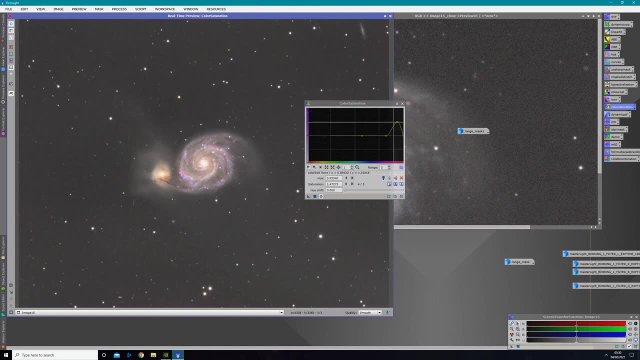 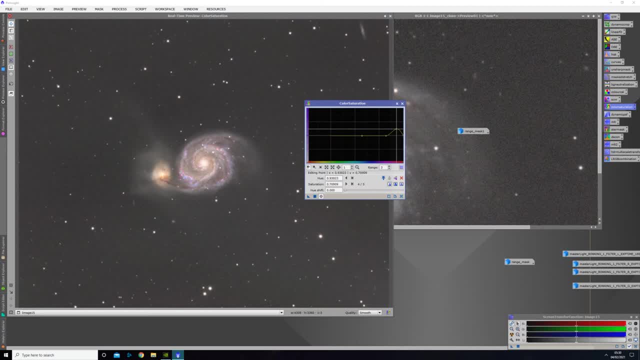 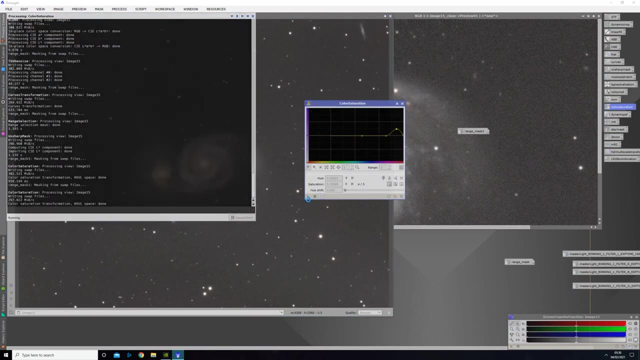 fine at this zoom. excuse it looks fine at this zoom. excuse it looks fine at this zoom. invariably gonna add quite a lot of noise that we don't want. so I think that's a nice gentle transformation. it still highlights the reds and doesn't introduce too much color noise. so I'm gonna go ahead with that, and so you may. 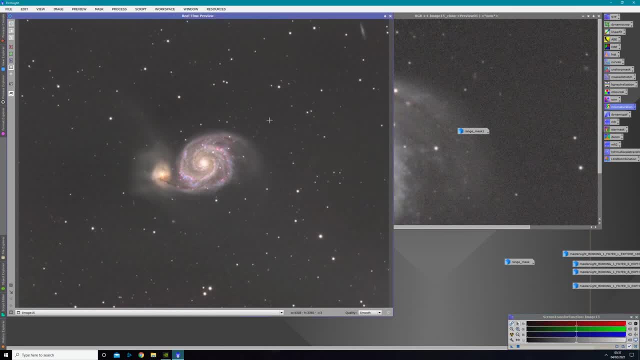 think I'm being quite muted with colors here, but it's just because I'm actually gonna de-stretch this image in a moment back to like a more pleasant level for my eye, and that's going to have the side effect of actually saturating the colors even further. so, again, we need the curves. transformation now close and 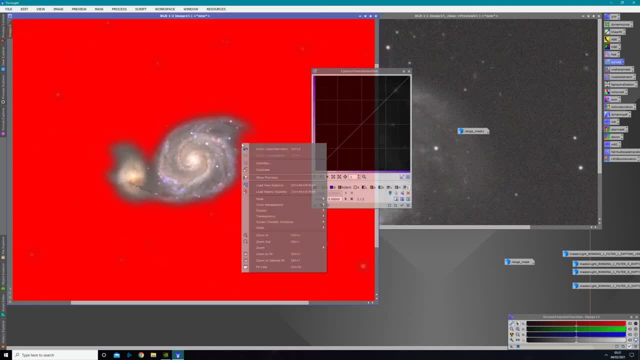 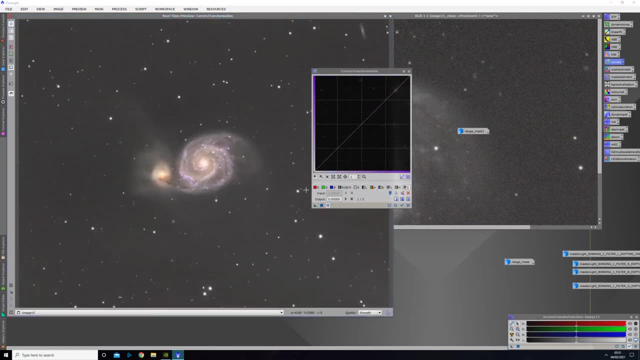 reopen a fresh preview. oops, sorry, before I do this, should add, I'm going to remove the mask, so I want to work on the whole image at once now. so again a preview. I'm going to skip select the RGB K part of the curves transformations, so as you. 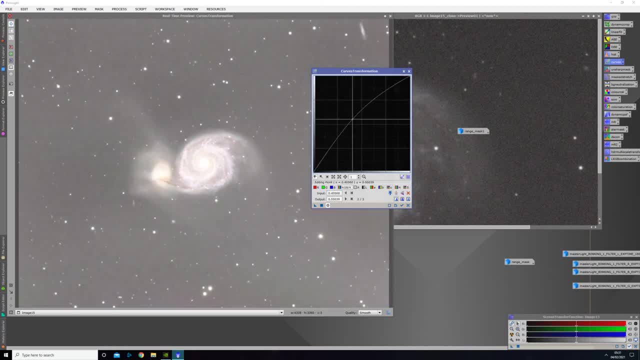 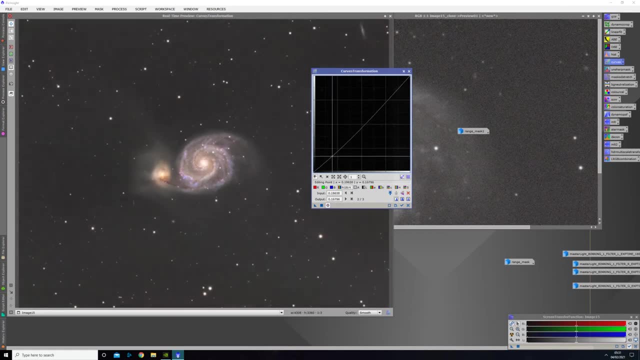 can see, if I grab the middle, push it up, things are gonna get blown out and down. they're gonna get crushed. so we need sort of a happy balance now. the further down to the bottom left of the Instagram you go, the further into the shadow tone as you're working, so I'm gonna actually try and drag this into a gentle s-bend. 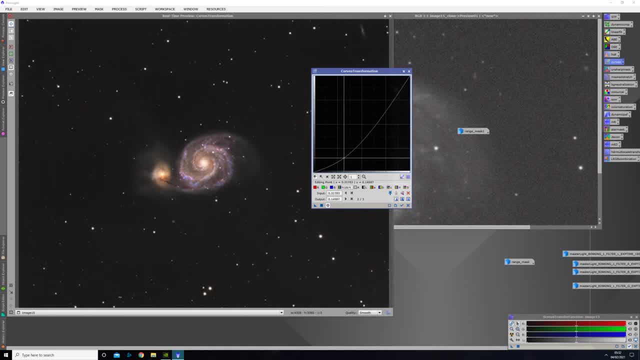 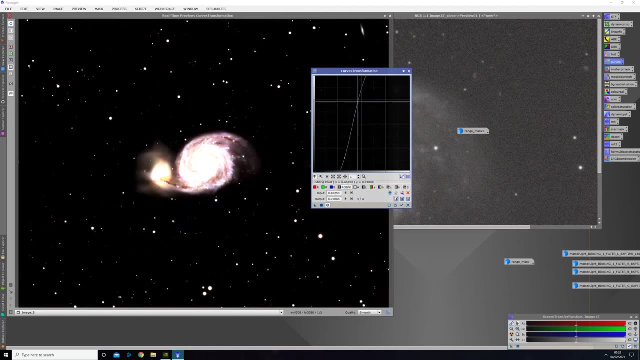 without going too dark on the background. so I think around about. there looks like a nice background level for my monitor and I- and I'm going to take the upper part of the histogram and just gently curve that back up. not too far, though, because if you grab all of this now and go too far, 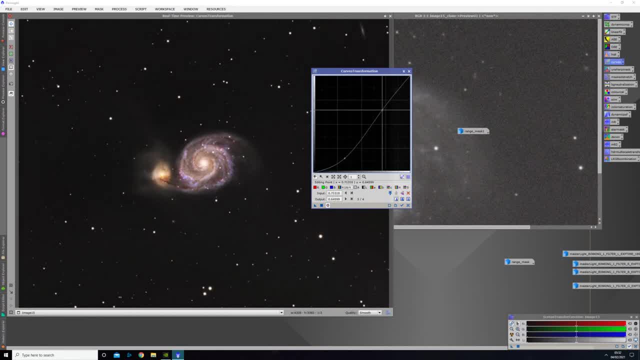 it's just gonna look awful. so before we apply that we can just check again that we're happy, and I certainly think it's an improvement. so I'm gonna add that and hopefully it shows that the color itself again has ended up further saturated just by doing this, or 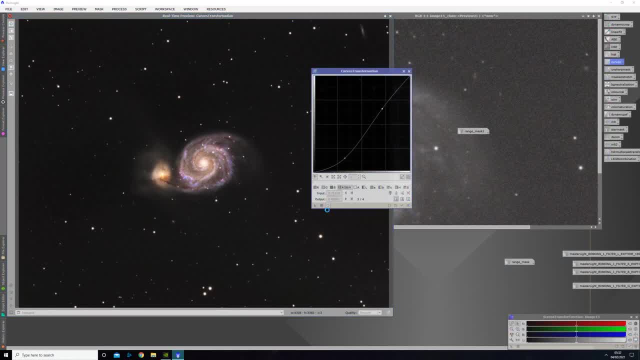 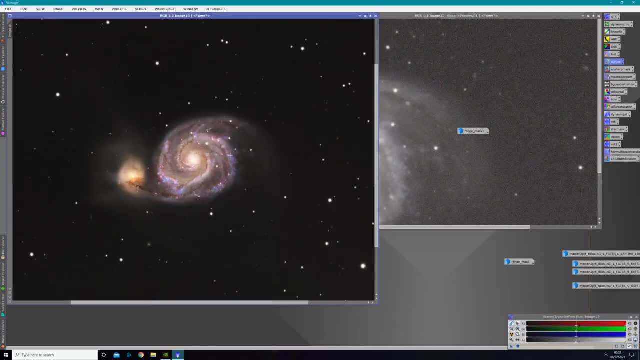 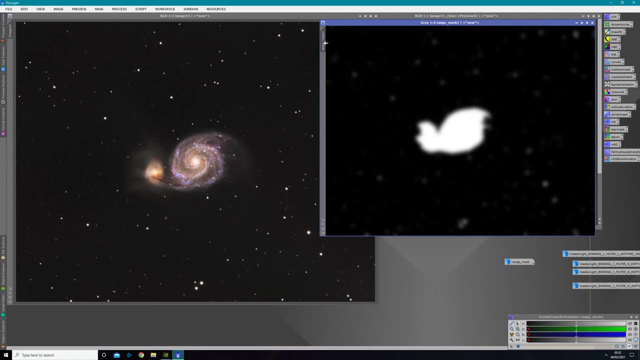 at least it's become more apparent. so I'll just reset the tool, close that down and we could call this largely processed now. but I think I'm gonna take the range mask that we had again, drop it on the image because I want to work on the. 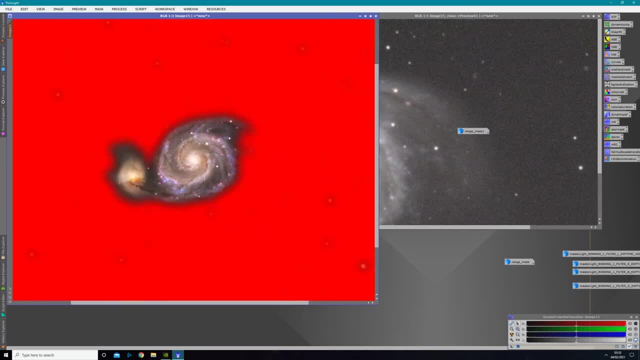 galaxy again. now we've added quite a lot of saturation. it's a has introduced some color noise, so I just want to go over this again with another pass of TGVD noise, this time maybe ever so slightly more aggressively as well, as we unsharp masked a little bit of extra detail, so